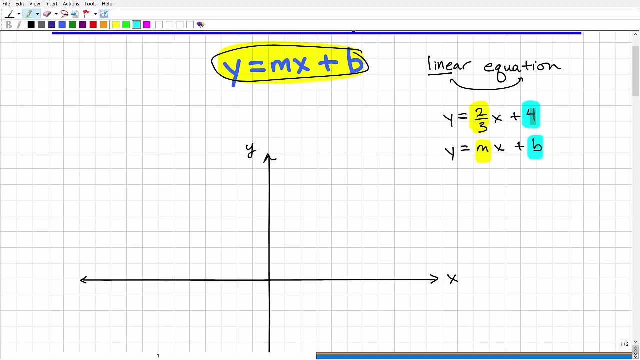 variable. in this particular example, the four is where the B is at. so basically it's Y equals some number in front of X, okay, which we call M. in this case it's two thirds plus another number. we're indicate actually plus or minus another number. okay, in this case it's for. so if you notice this line here, this linear, 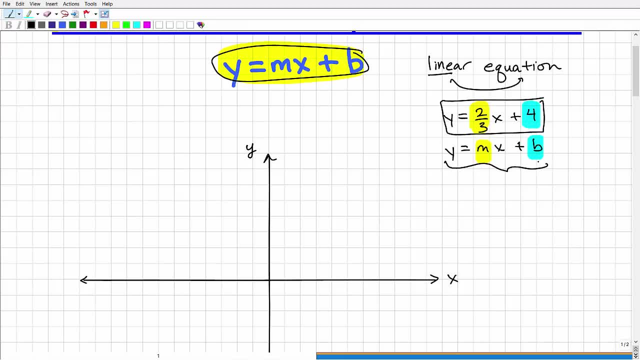 equation follows this format. so when you're looking at a linear equation or an equation and it follows this line here, if I enter this line in the first equation- equation of a line- okay, then we can actually graph it pretty easy, Okay. so let's go ahead and just 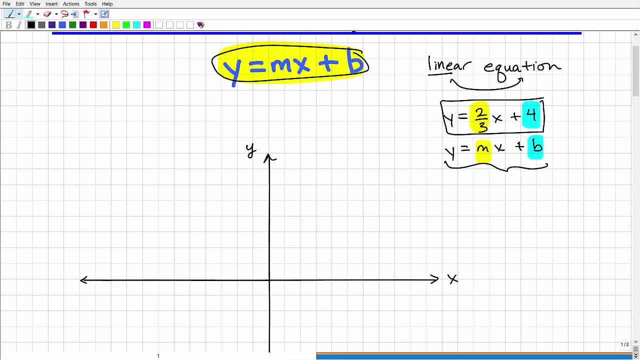 work through some problems, put a little variety in them. you know we'll do a few different types and this doesn't have to be all that difficult. Okay, so what's the first step we do? Well, let me just back up and say this In order to graph a line, right, I want to put some sort of line. 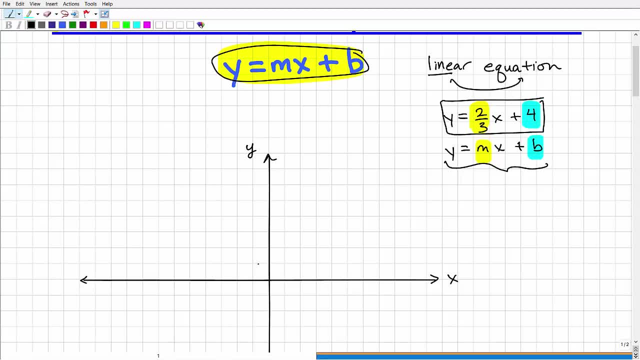 on my graph or graph it, and you can see here I'm going to have graph paper already kind of set up in my video. You need two points. so I need like a point here and I would need one other point that's on that line and I'd be like: okay, these two points are on the line. so therefore I can. 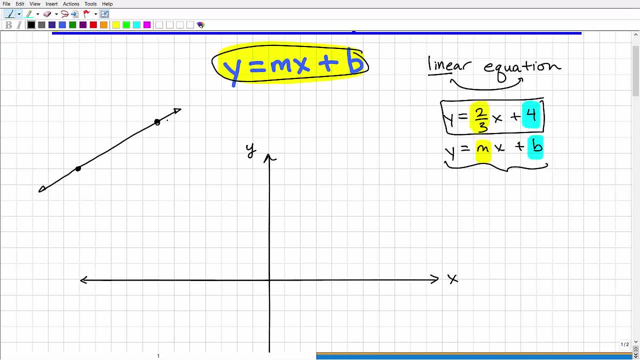 draw or sketch the line right, because the line would go through those two points, and then you have the graph of that line. So that's what we're going to be doing here. The whole idea of graphing a line using the y equals mx plus b. 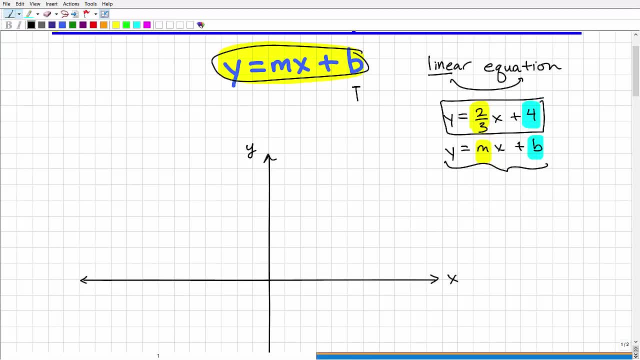 format. it's really easy. The b number is our first point. okay, that we're going to plot Now, for example, maybe like right here and that's not there, but I'm just you kind of get the idea. 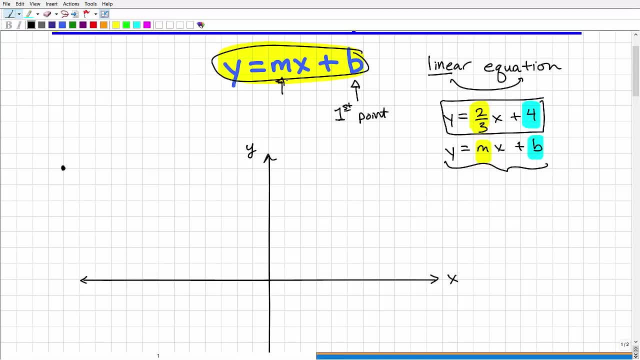 right, so we'll have one point, and then the m number gets us to our second point. All right, so let's say that's like right there. So once we have two points, then we can graph the line. All right, so we just need two points, and these two points are going to be on the line. 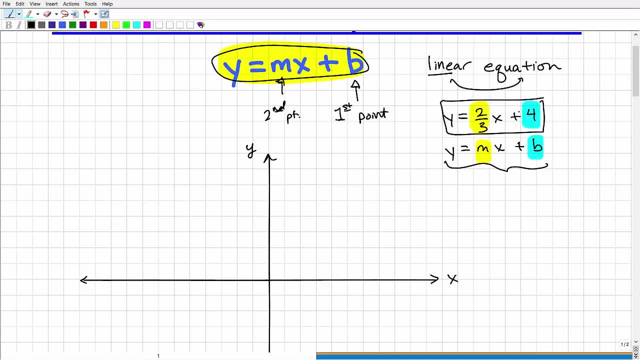 All right, so let's start off with the first point, and that's the b value. This is really really simple, okay? So let's look at this In this example. it's four. The b value is what we call the y-intercept, and all that means is where the line is going to intersect the y-axis. So 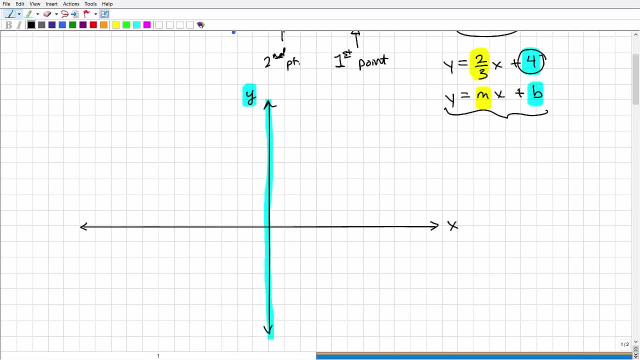 this is the y-axis right here, So this particular line will chop through or intersect the y-axis at four. So you just basically count from zero up to four, and I'm assuming you have basic knowledge of the coordinate plane. If you don't, then you'll want to review that for this video. 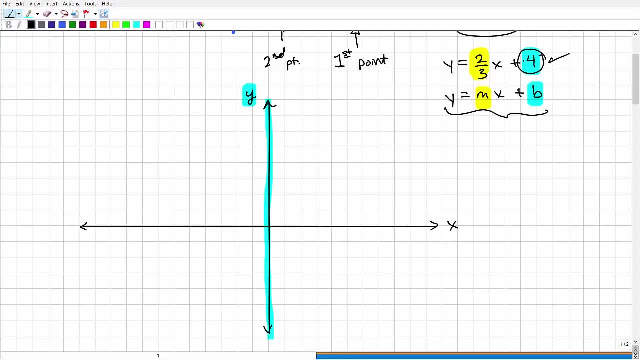 but this line is going to cross the y-axis at a positive four. So we just go up to positive four on the y-axis. one, two, three, four and that is our first point. Very simple and, like I said, this does not have to be overly complex. So we've got one point. that's on the 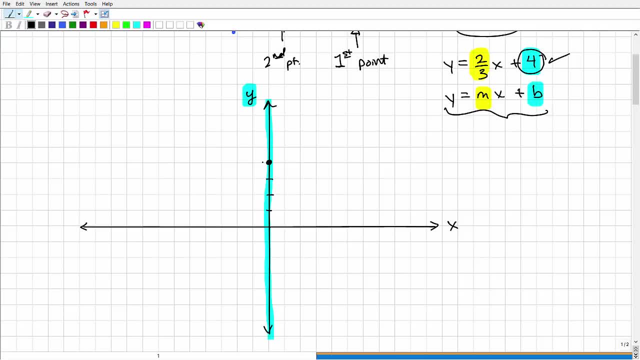 line. and now we need that second point, that we can graph the line. So this is where students tend to get confused. okay, Now let's talk about the slope. Now, the slope of the line here is two thirds. all right, I'm going to write this over here: two thirds, and I want you to kind of 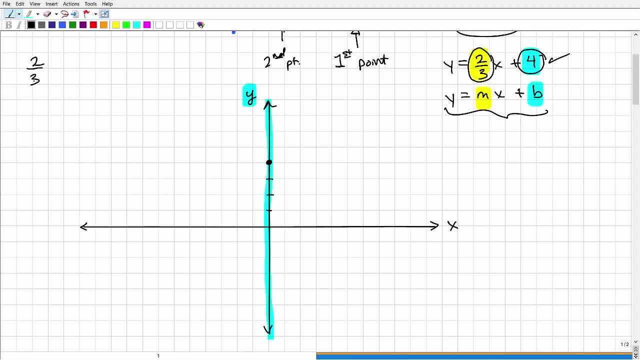 remember the following: okay, The slope of a line, when we plot it using y, equals mx plus b. it's either going to go up and to the right or down and to the right. okay, If the slope is a positive number, we're going to count up and to. 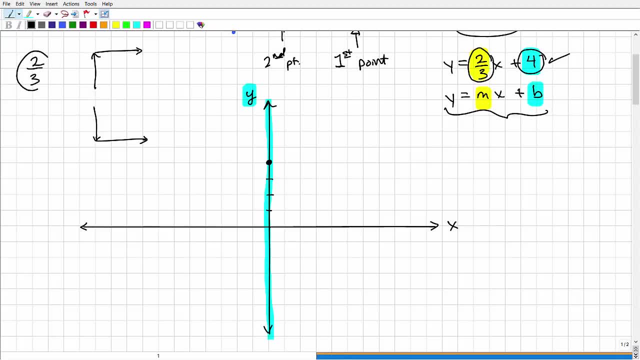 the right. So in this case, two thirds is positive. Now I'm going to show you what I'm going to be counting here in a second. okay, If, for example, this was a negative two thirds, I would be going down and to the right, but always to the right. We're going to be counting always to the right. 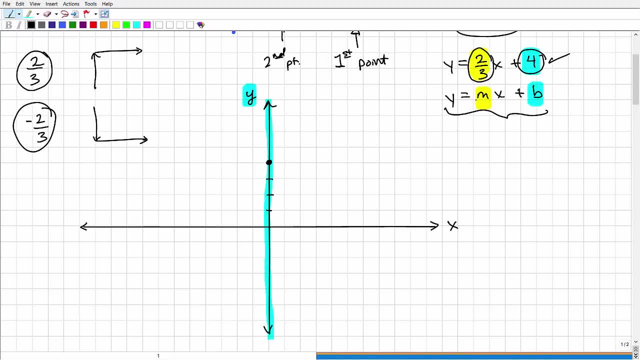 and if the slope is positive, the m value is positive, we're going to go up. If it's negative, we're going to go up. If it's negative, we're going to go down and to the right. And we'll look at another example here in a second with a negative value. Matter of fact. 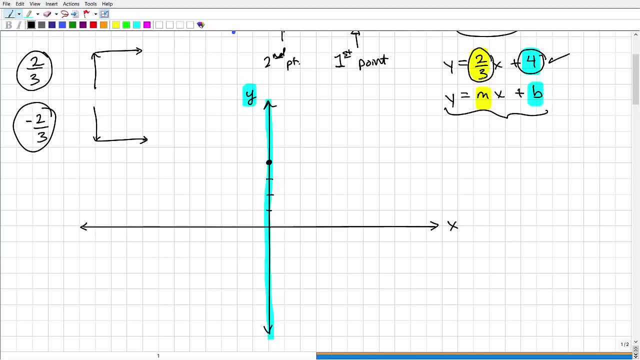 we'll do the same, one kind of tweak it up a little bit. Okay, so now, what do I do? Okay, now, like, how do I, you know, manage this number? I'm not going to try to overly explain this in. 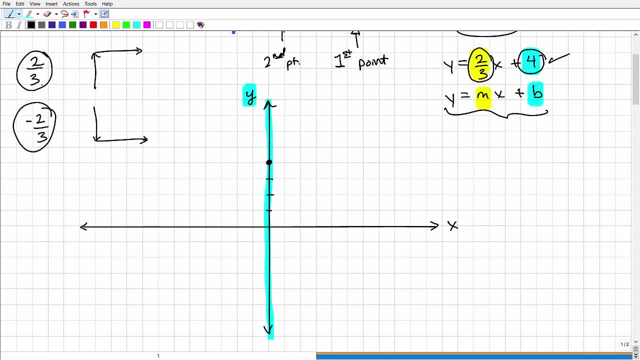 terms of getting into the slope in too much detail right now, because that's the purpose of this video. I just want you to be able to grab the line. So here's what you're going to do. This top number two is how much we go up and to the right. So I'm going to go down and to the right And I'm going to. 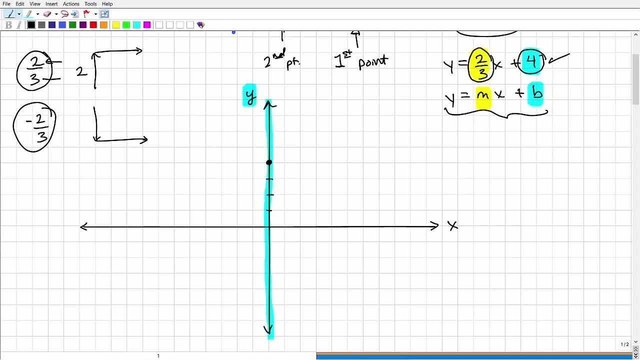 go up. So we're going to count up two And this number here, the bottom number we got, the denominator is how much we go to the right. So the slope, this, the slope here, this two thirds, is kind of like a driving directions to our second point. you're going to go up to and to the right. 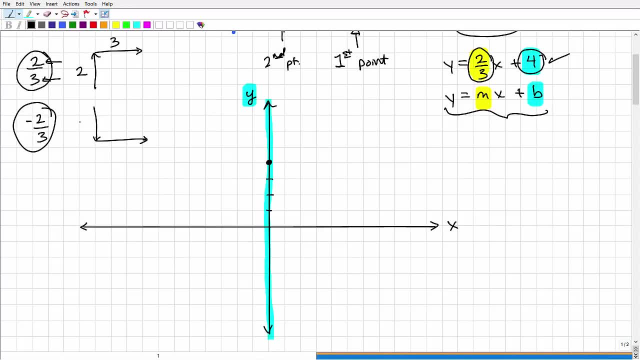 three. Okay, if it was negative, we would go down to okay and to the right three. okay, in this direction, a negative direction. So here's how we do this. Okay, starting from the y intercept. okay, we're going to go ahead and count up to and to the right three. 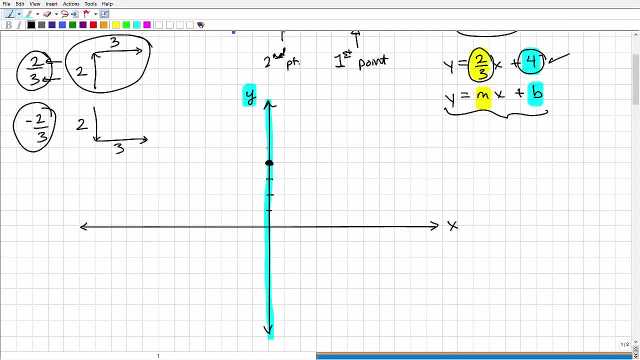 because this is a positive slope. So from here we're going to go up to 12.. All right, you can see, I just went up to, and now I'm going to go right- 3123. And that is where my second points at. Okay. 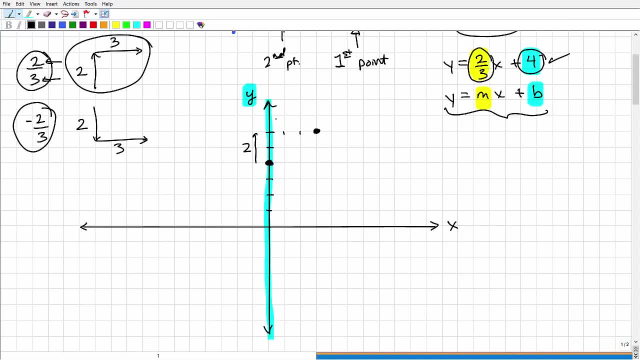 so I went up to here All right, And I went right three. That's all I did. And then all I do is just draw my line through these two points and I'm done. I'm just kind of sketching in here, but you get the idea. So this line has the equation: y equals two thirds x plus four. 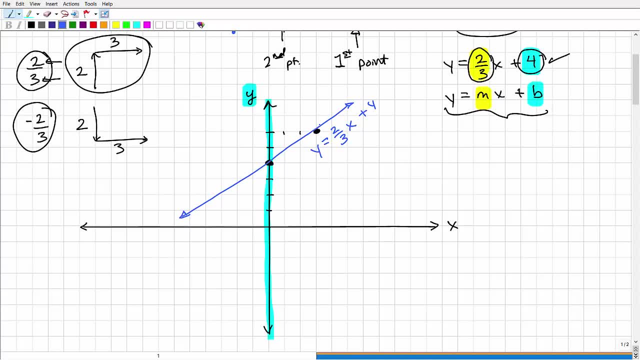 this is the linear equation to this line. Okay, That's why you know, when you have a line in y equals mx plus before, it's so easy to to graph. So let's go ahead and take a look at some other things here. All right, let me erase this And let's let's go over here. Let's actually matter. 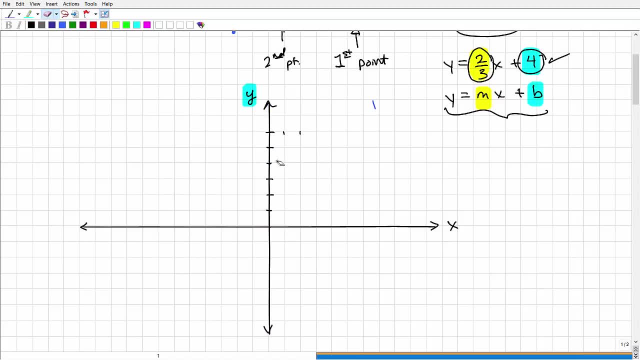 of fact, I'll give you a chance to see if you can actually figure it out. Okay, So let's, let's use this same example. Let's change this up a little bit And we'll make it y equals. let's do it this. 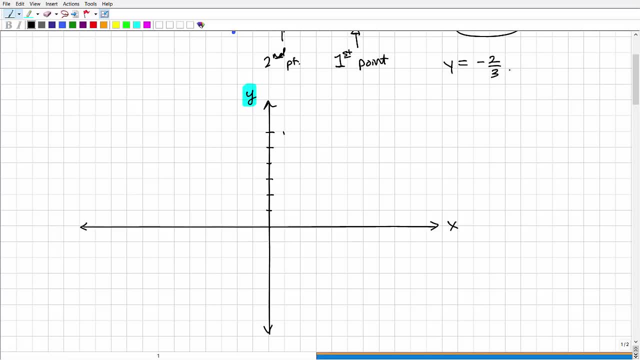 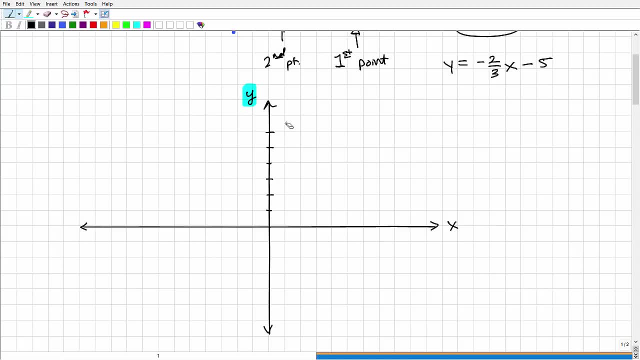 graph that All right. so maybe you want to pause the video and give it a shot? Okay, so let's take a look at what we do Remember. the first thing is we look at the b value. In this case it's. 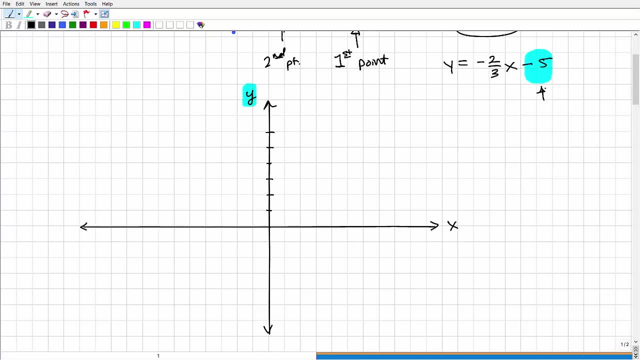 negative five. we start here And we count on the y axis on this, to this, to this value, okay, this number. So on the y axis, the negatives are this way: Okay, so I have to go down five: 12345.. So that's. 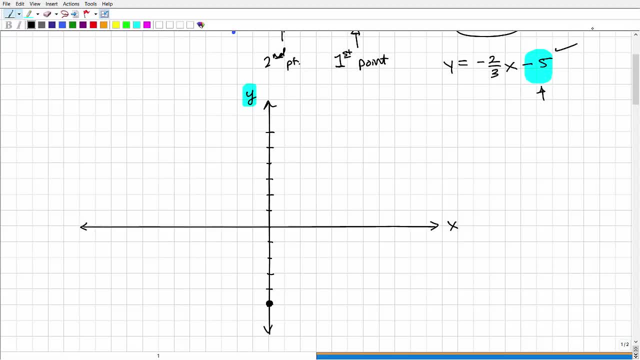 my first point Very simple: Okay, that's on a line Now. Now, from there, I got to take a look at my slope. Now this is a negative slope, So that, therefore, it's going to go down and to the. 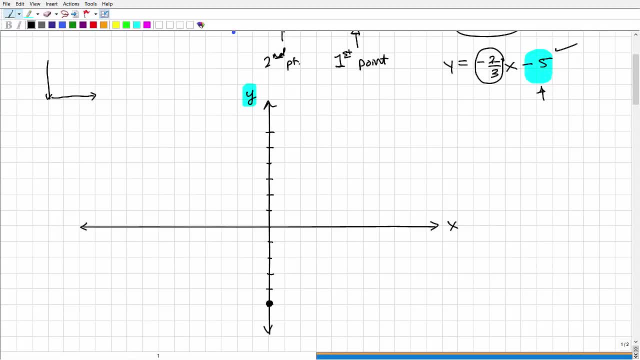 right, Okay, but down how many? Well, the top number tells you how much it's up or down. the bottom numbers always To your right. So it's going to. we're going to count down to and to the right three, So let's go. 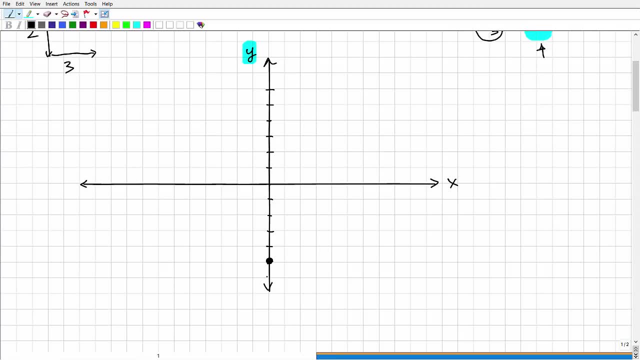 ahead and do that. We'll give ourselves a little bit more room. So one, two and then, to the right, three, 123.. And that is our second coordinate for this line, And then we just go ahead and draw our line through it like so And that is it. Okay, that's how you graph lines is using y equals mx. 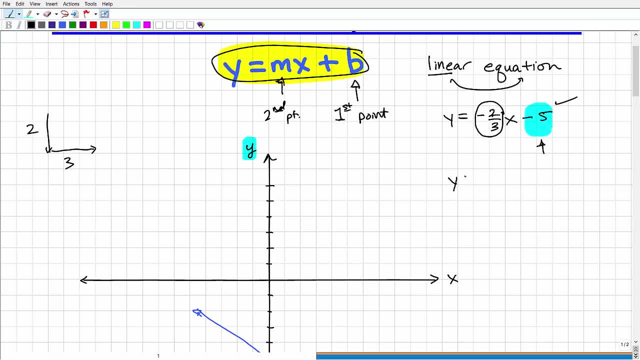 plus b. Now let's take a look at it. Another example: I'm not going to actually graph it, but let's take a look at something like this: y equals three, x plus seven. Well, you might be saying: okay, well, this is seven. I know I could count up 1234567.. There's my first point. But you might be. 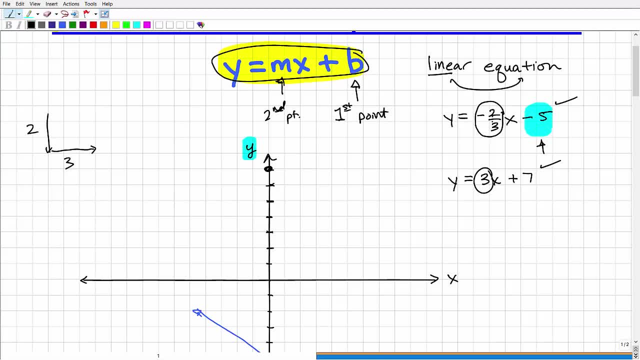 a little confused about that slope. You're like: well, three, what? I don't see the fraction there. Remember, if you have a whole number, just put it over one. three over one. Okay, now you can see it clearly. Okay, so what am I going to do here? this is going to be up three over one, up three.